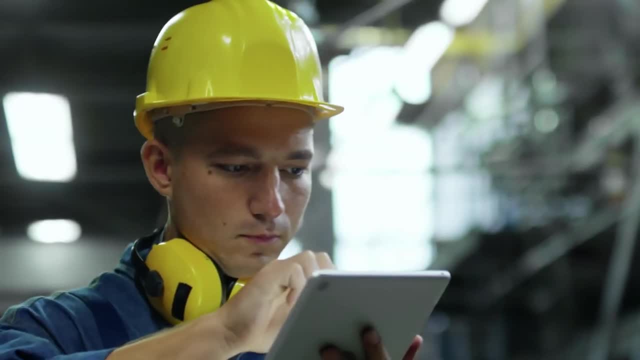 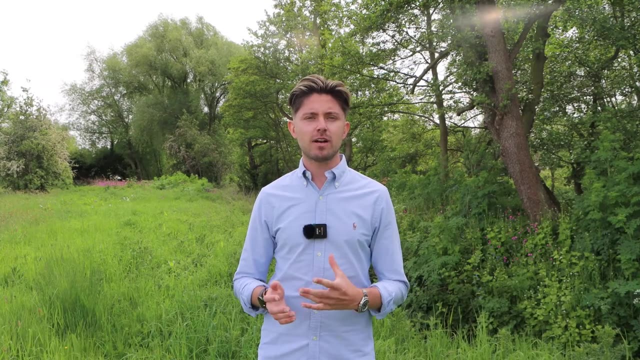 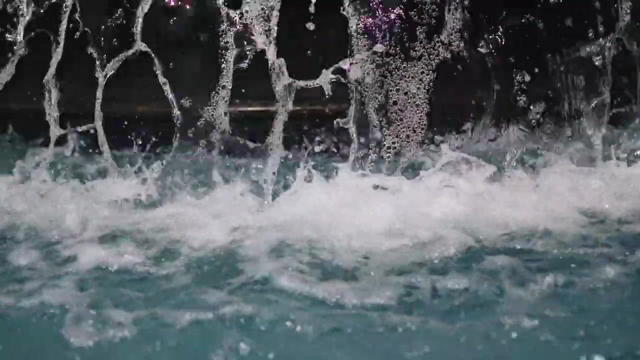 site from all of these sources and, where feasible, provide recommendations for mitigation measures to alleviate the impact of flooding on a site and its surrounding area. An FRA is generally required to be submitted as part of a planning application for all potential site developments proposed in flood risk areas. It's critical for developers to understand the potential flood risks. 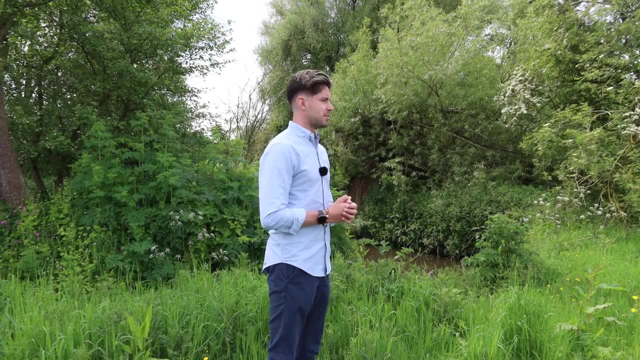 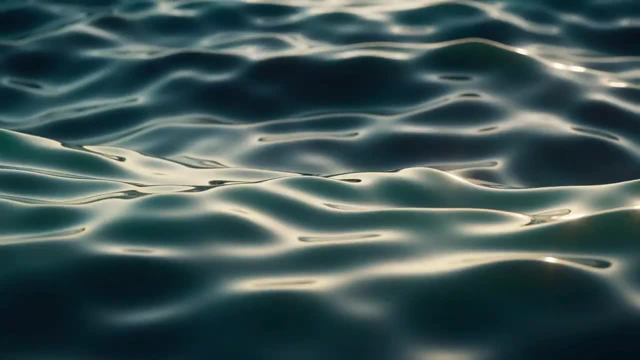 to a new development, not only to determine the safety of the development in relation to the flood risk, but also to understand the impacts the development may have on surrounding areas in terms of increasing or exacerbating flood risk. The aim of a flood risk assessment is to find out. 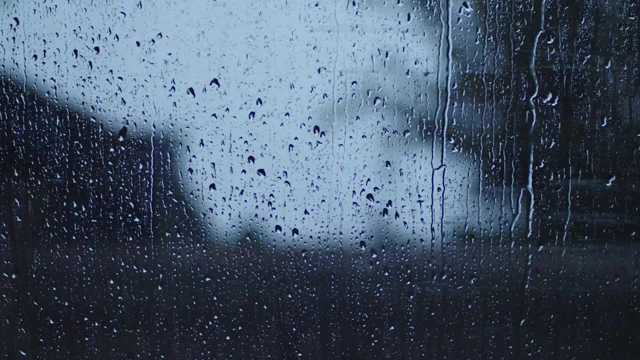 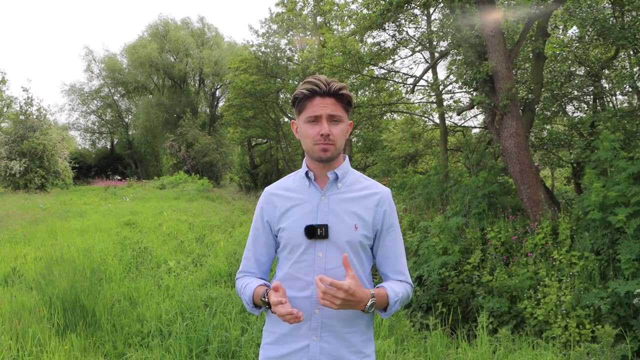 whether the proposed development is likely to be affected by current or future flooding from a range of sources. whether the development will increase flood risk elsewhere. whether the mitigation measures proposed to deal with the potential flood risk are appropriate. whether the development will be safe over its lifetime. 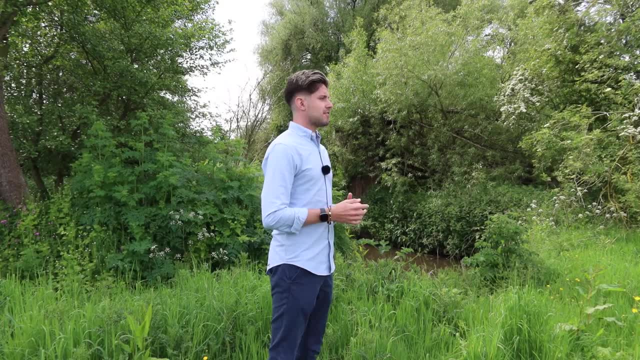 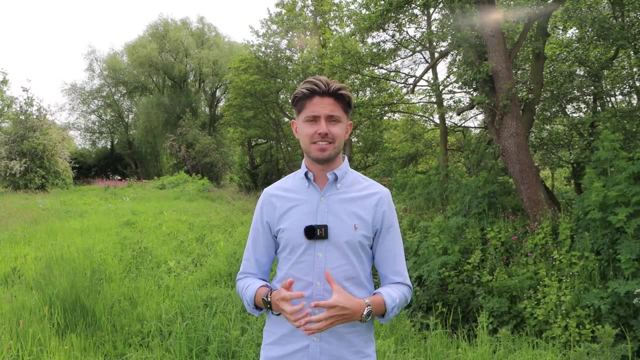 So do you need a flood risk assessment? Requirements for an FRA differ between Scotland, England and Wales, where planning matters are devolved. A flood risk assessment in England is required when the proposed development is located within flood zone 2 or 3 or 3 or 3.. 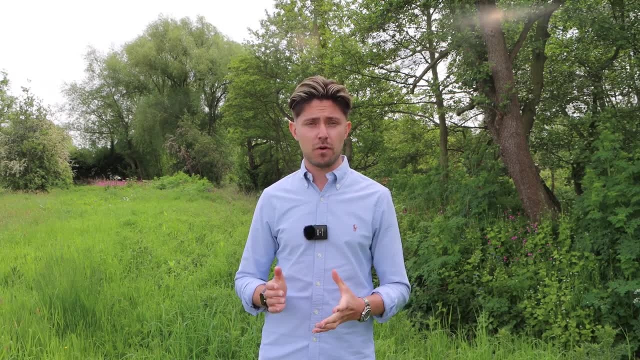 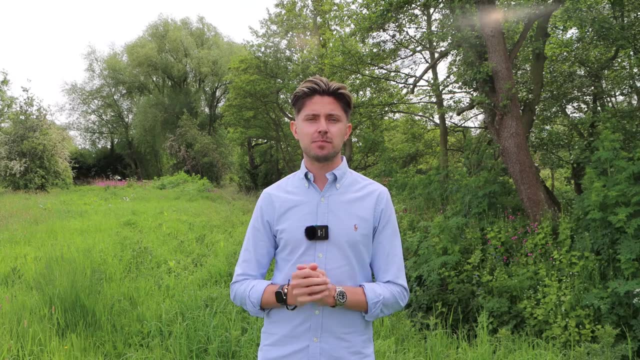 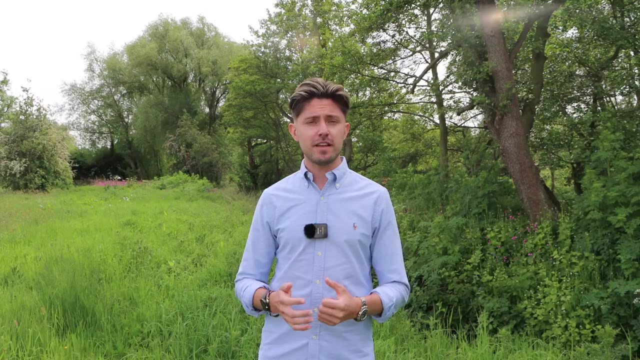 the site is located within flood zone 1 but is greater than 1 hectare. or the site is located within flood zone 1, is less than 1 hectare, but is affected by other sources of flooding, such as surface water or groundwater or sewer flooding. So what are flood zones? There are three flood zones as defined by the. 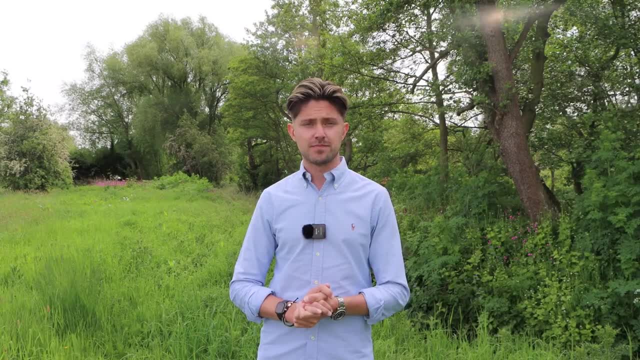 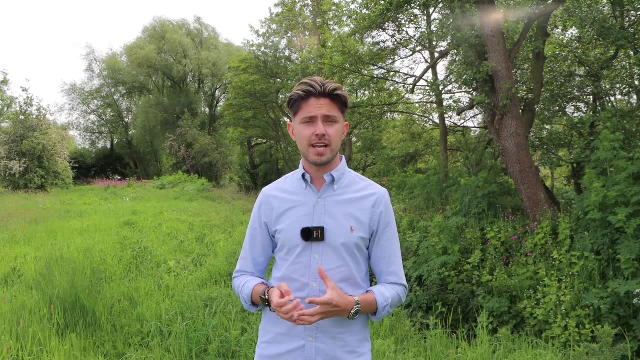 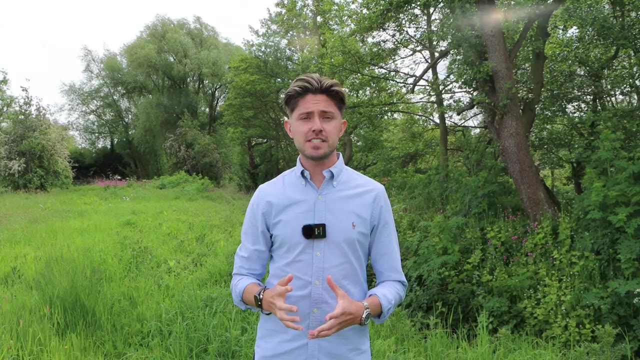 Environment Agency. flood zone 1,, 2 and 3.. The flood zones are based on the likelihood of an area flooding from rivers or the sea and for catchments greater than 3 kilometres squared with flood zone 1- areas least likely to flood, and flood zone 3- areas more likely to flood. These flood zones do not always. 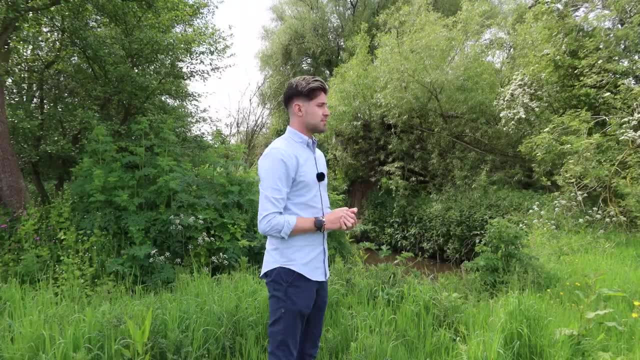 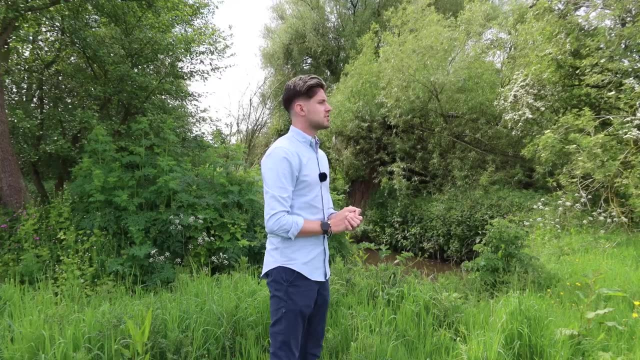 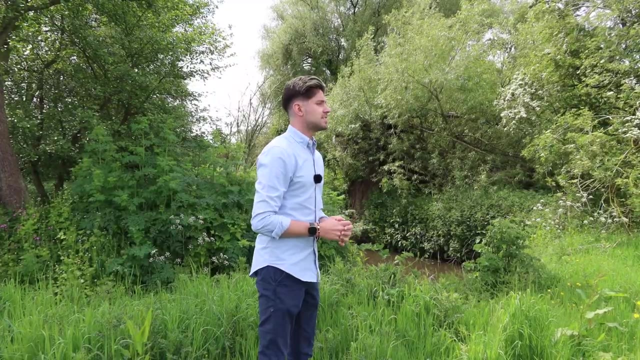 consider every single river in an area and don't consider blocked drains, nor do they currently take into effect the effects of climate change. Therefore, sites shown to be in flood zone 1 can still experience flooding, and surface water should not be ignored. Areas within flood zone 1 are deemed to have less. 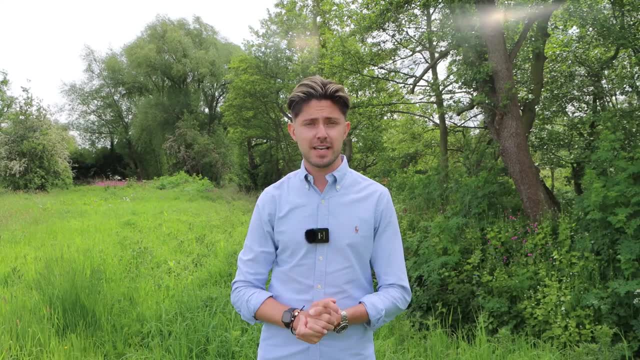 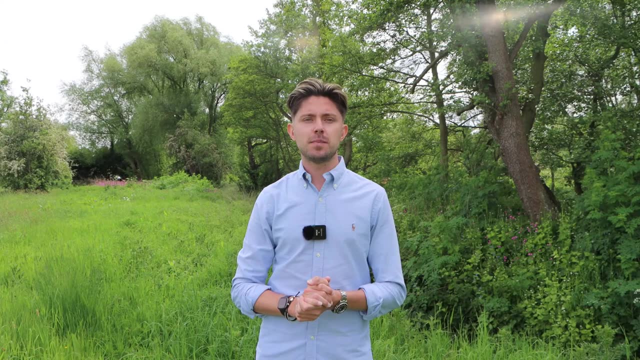 than a 1 in 1,000 or nearly 1 in 1,000 flood zones per year. There is a 0.1 percent annual probability of flooding in any given year and flood zone 1 is the lowest risk flood zone. There are typically few restrictions in. 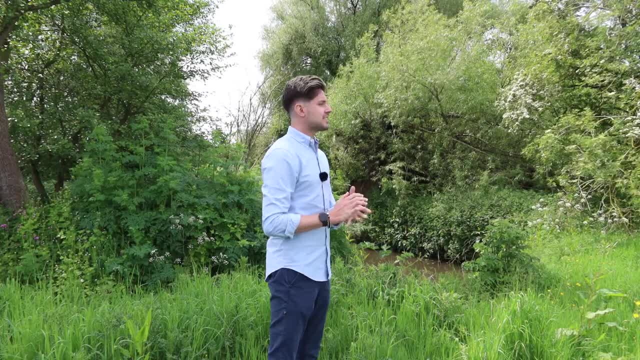 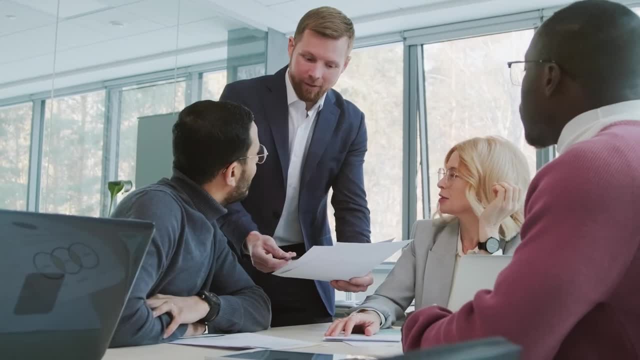 terms of flood risk to development in flood zone 1 areas, and the exception is for developments over 1 hectare in size, which must have a flood risk assessment undertaken as part of a planning application, and areas deemed to be at high risk of flooding from surface water, known as critical drainage areas. Areas 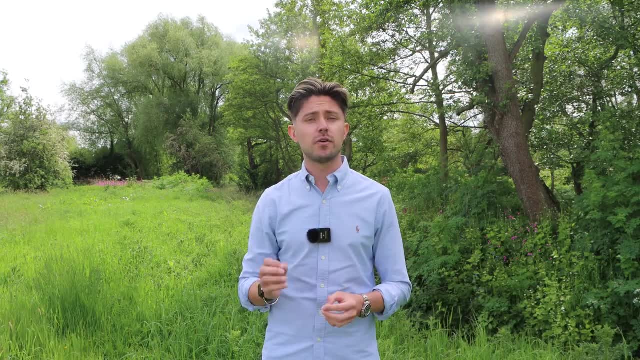 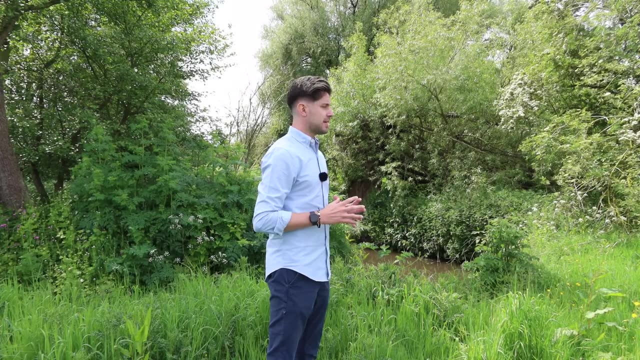 within flood zone 2 have between a 1 in 1,000 or 0.1 percent and a 1 in 100 or 1 percent annual probability of flooding in any given year. Flood zone 2 is considered a medium flood risk Development situated. 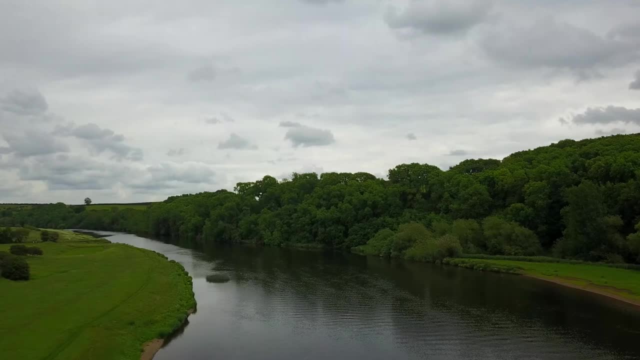 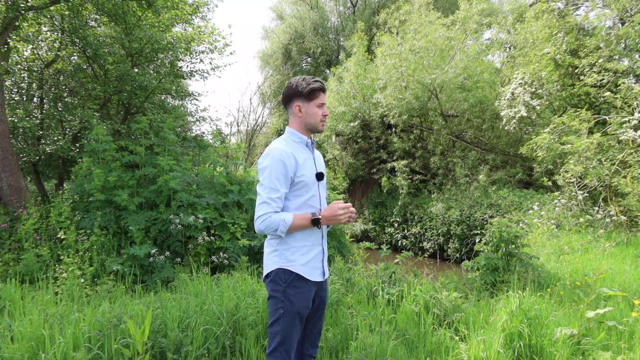 within flood zone 2 require a flood risk assessment to be submitted as part of any planning application showing the risks of flooding to the site. Flood zone 3 is split into two separate zones, 3a and 3b, by the local planning authorities. 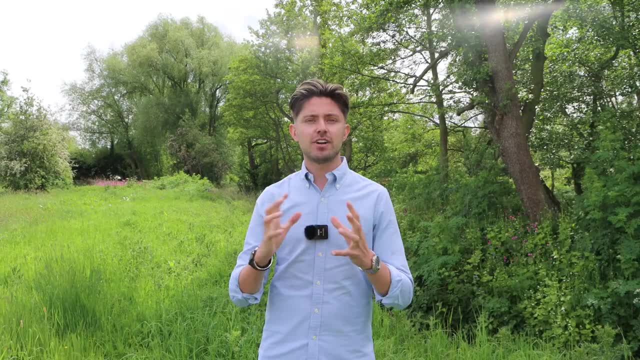 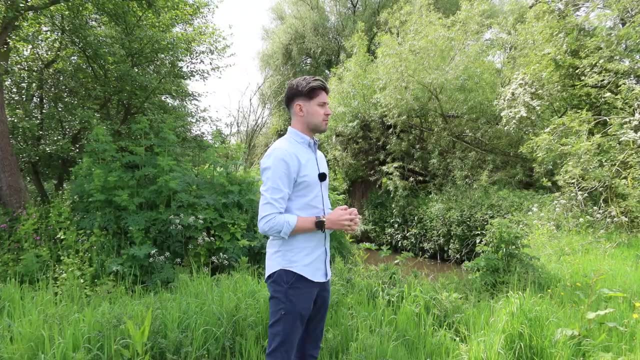 However, flood zone 3 areas appear as a general flood zone 3 area on maps, Due to the EA not splitting these zones. areas within flood zone 3a have a 1 in 100 or 1 percent or greater annual probability of flooding in any given. 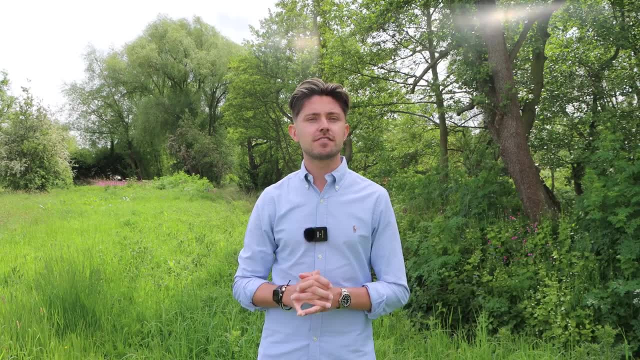 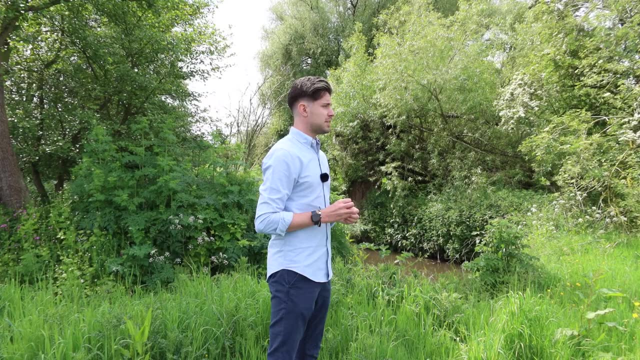 year. Flood zone 3b are areas classified as functional floodplain and are deemed to be the areas at most risk of flooding. Areas located within flood zone B typically have a 1 in 20 or 5 percent chance of flooding in any given year. 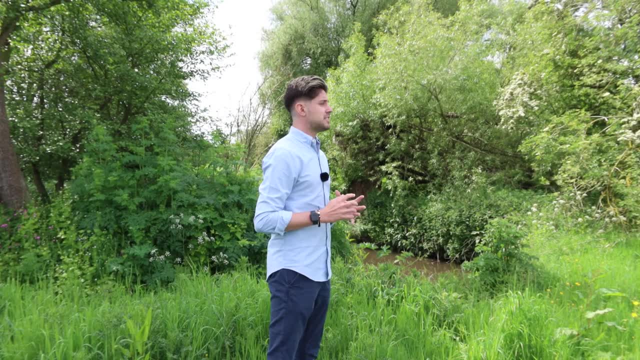 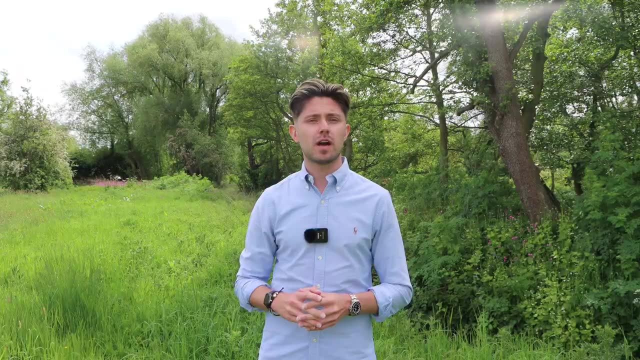 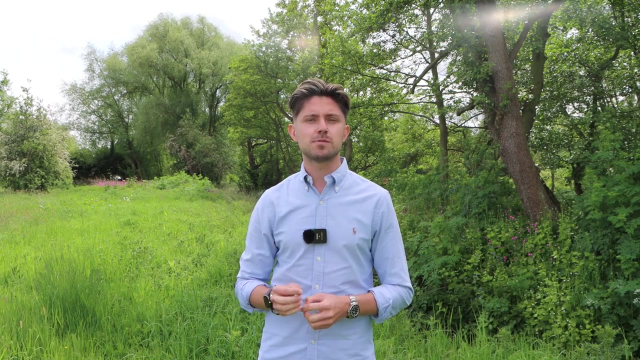 There are significant restrictions as to what can be developed on flood zone 3a. It is extremely important to know whether you require a flood risk assessment to accompany a proposed development, for both safety and legal purposes. The last thing you want is your proposed development displacing water. 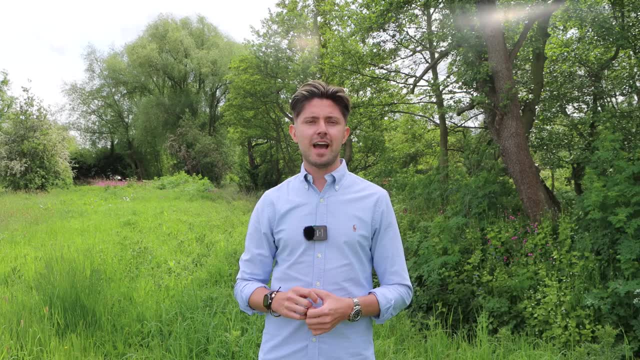 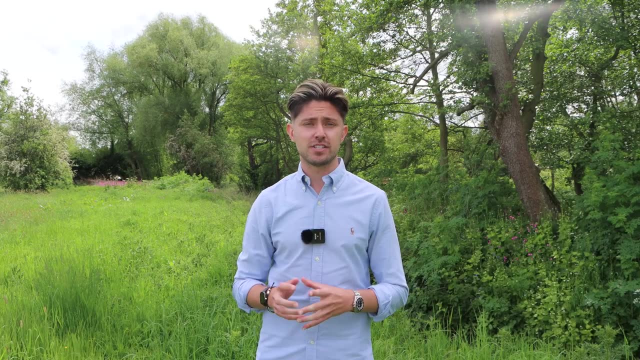 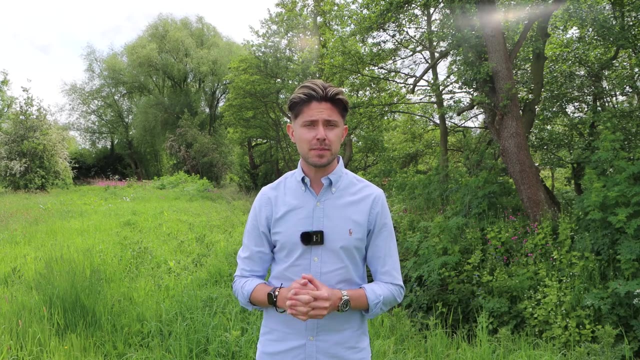 and someone using this to make a claim against you. We have an extensive background and extensive experience undertaking flood risk assessments to support planning applications across a range of properties, flood zones and development proposals. Our flood risk assessments use the most up-to-date and high-tech data available, combined with working 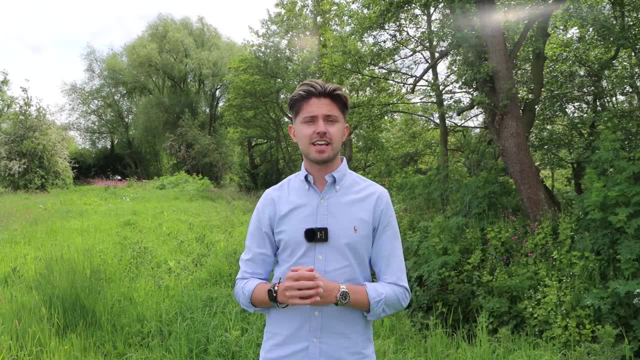 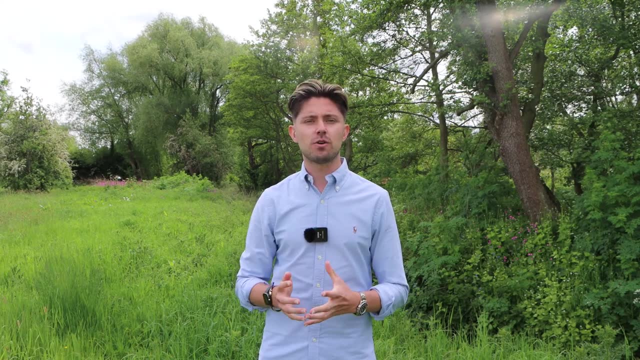 collaboratively with a range of organisations and sectors, such as the Environment Agency, architects, lead, local flood authorities and with the client themselves. If you're unsure and need advice, please get in touch with our team of specialists.